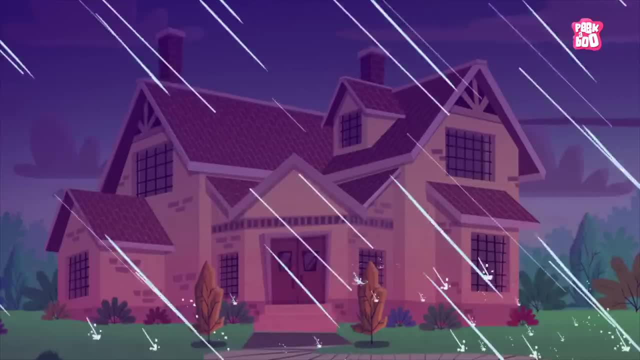 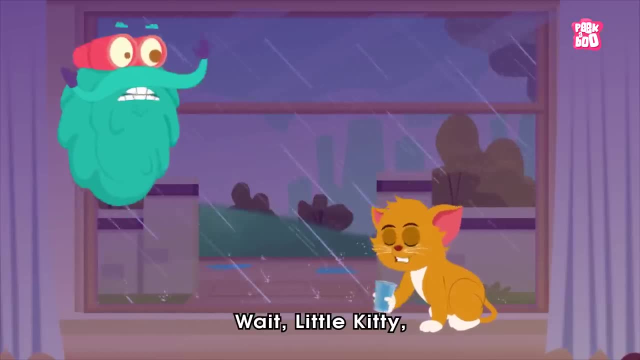 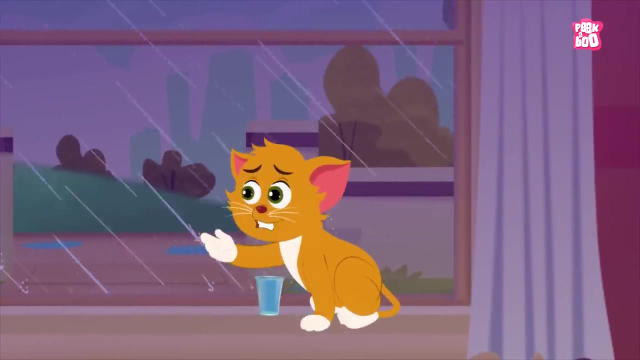 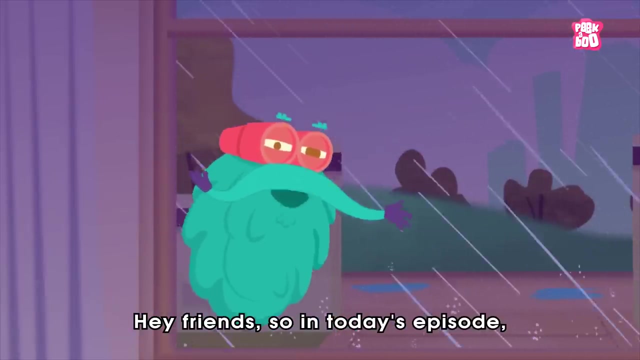 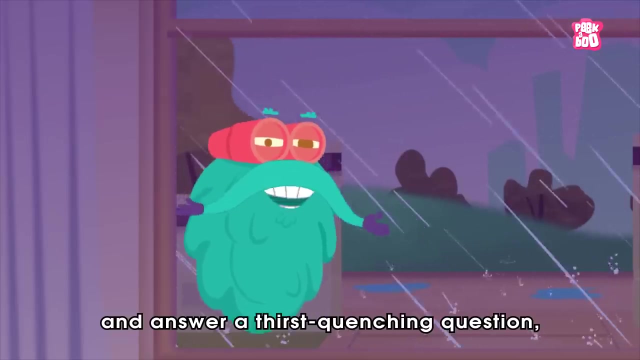 Wait, little kitty, before you drink that rainwater, make sure you know how it's formed, How Well, that is what I'm here to explain, Hey, friends. so in today's episode, let us have a microscopic look at the rainwater and answer a thirst-quenching question. 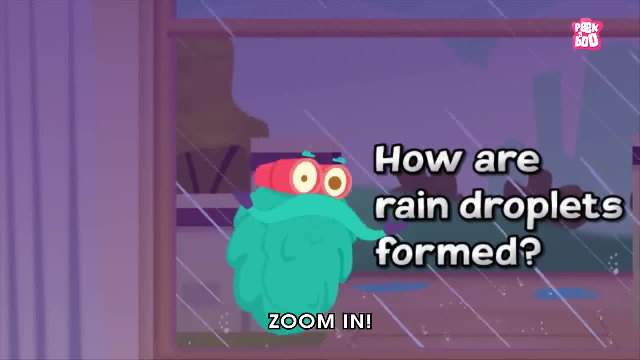 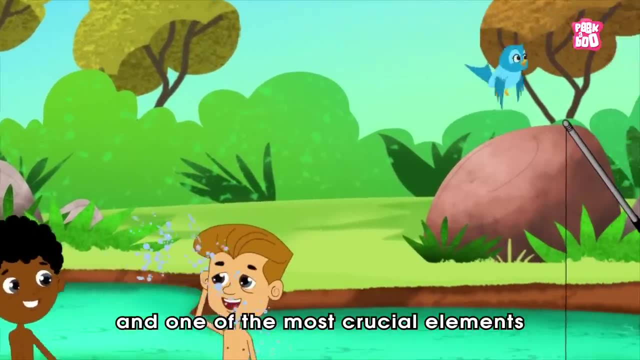 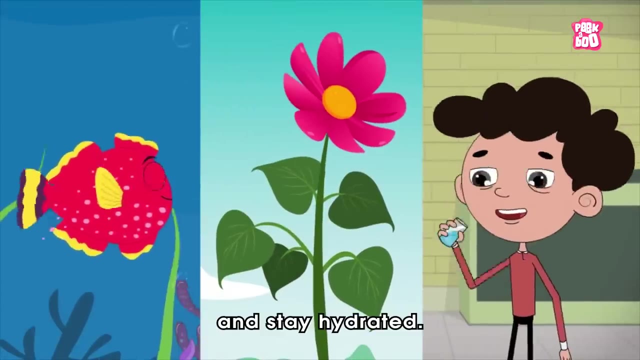 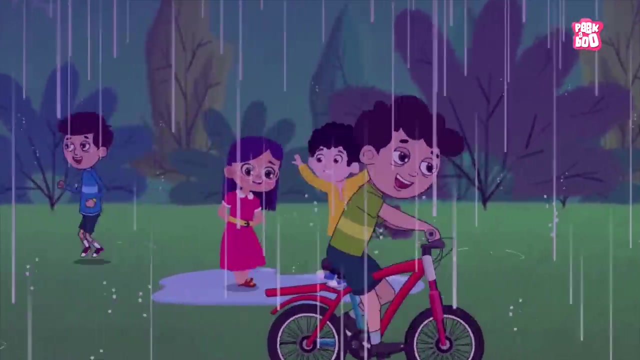 How are rain droplets formed? Zoom in Water, the reason behind our existence and one of the most crucial elements. all living beings need to survive, grow and stay hydrated, And the best part is Mother Nature has provided it for us for free, in the form of rain that falls from the sky through. 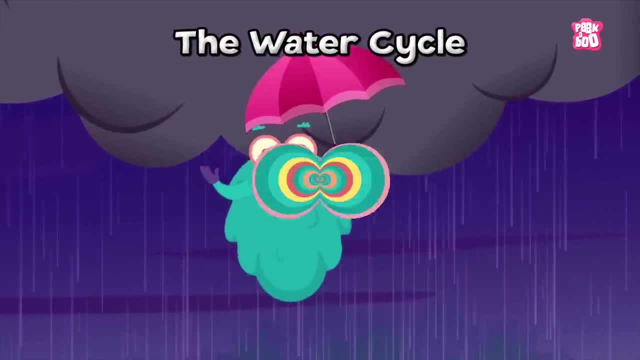 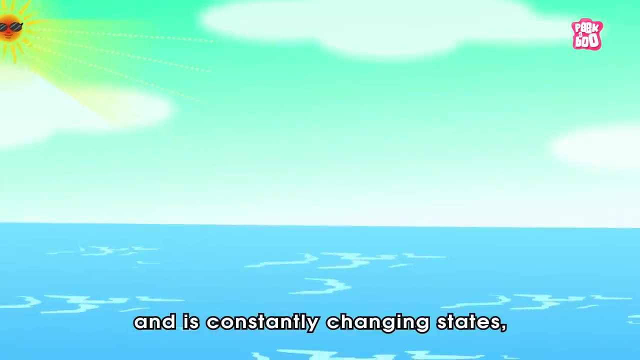 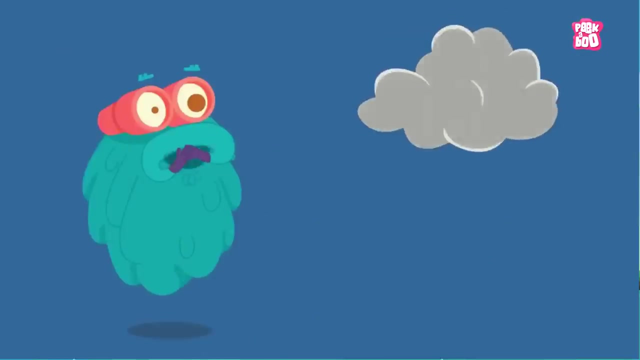 a process called the water cycle. The water cycle explains how Earth's water is always in movement and is constantly changing states, from liquid to vapor, to ice and back again. And if you are not aware of it yet, then don't forget to subscribe to our channel by clicking on the bell icon. 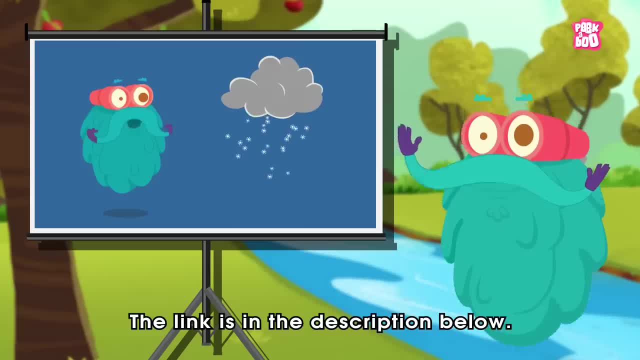 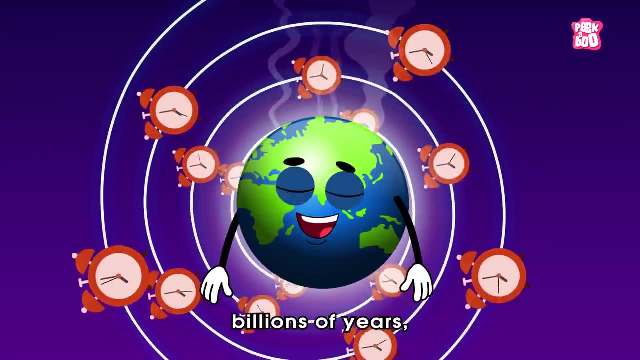 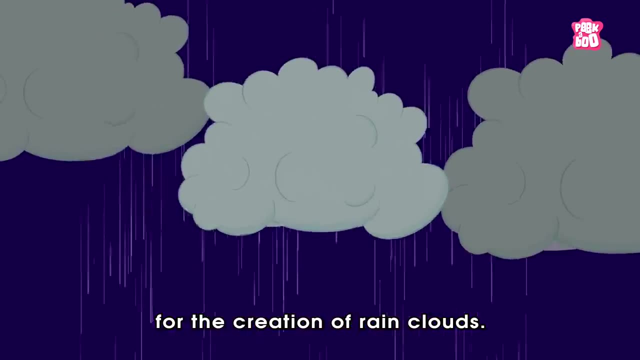 And do check our video on the same topic. The link is in the description below. Although the water cycle has been working for billions of years and most of us are aware of the fact that how crucial it is for the creation of rain clouds, However, when it comes to the 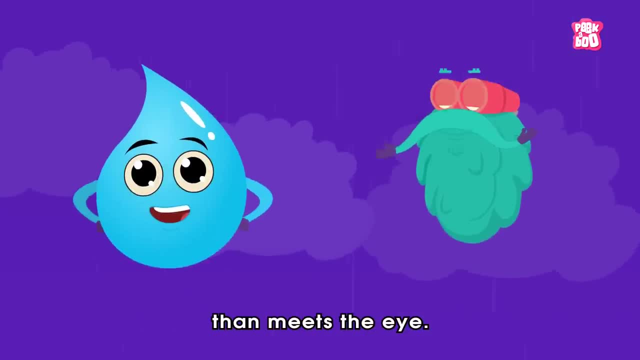 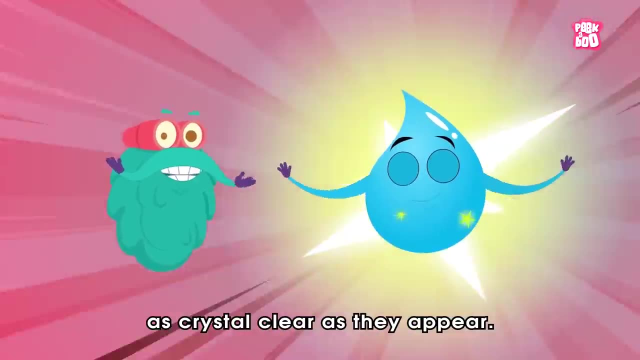 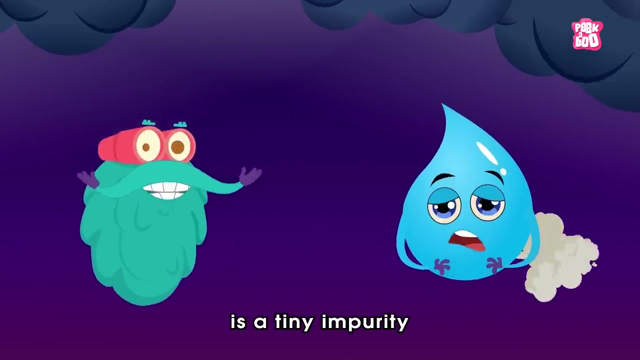 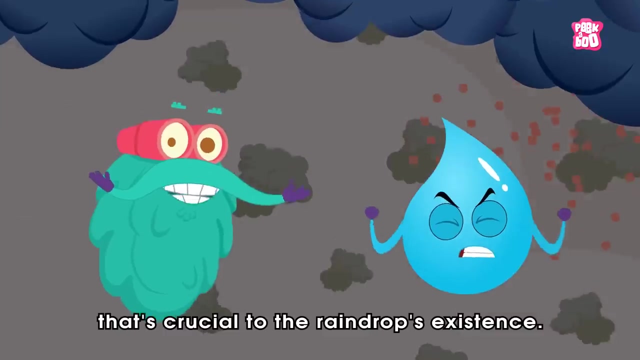 formation of rain drops. there is more to it than meets the eye. Yes, my dear friends, rain drops are not always as crystal clear as they appear. Somewhere inside of every raindrop is a tiny impurity consisting a touch of salt, a speck of soup, a grain of clay that's crucial to the 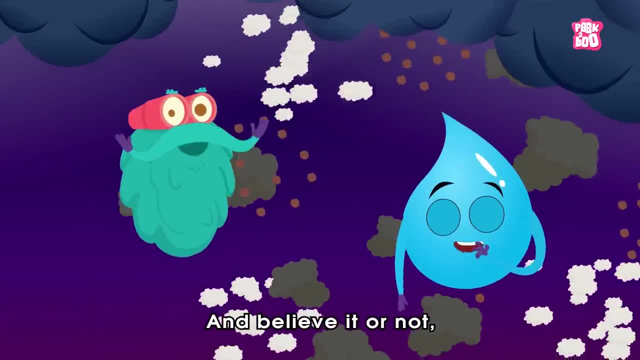 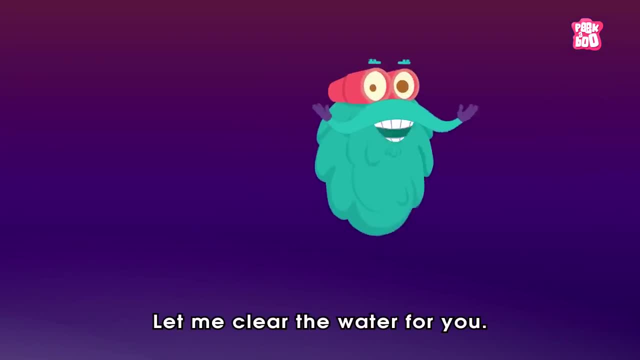 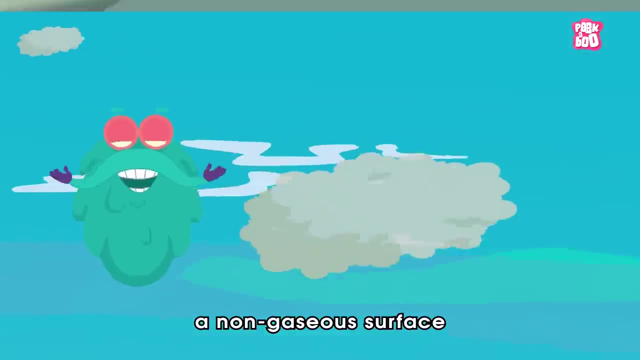 raindrops existence And, believe it or not, without these impurities there would be no rain. Confused, Let me clear the water for you. You see, water requires a non-gaseous surface to make the transition from vapor to a liquid. 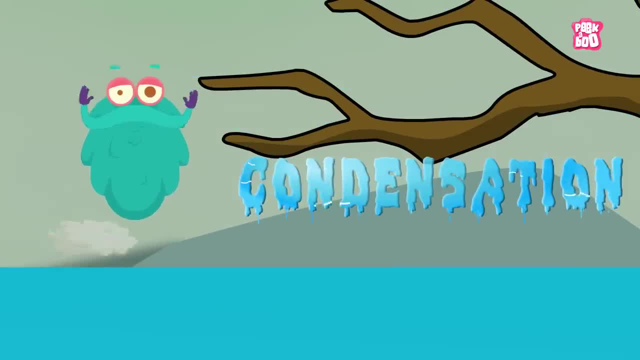 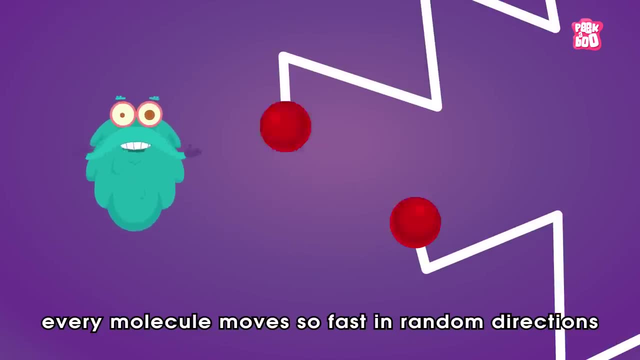 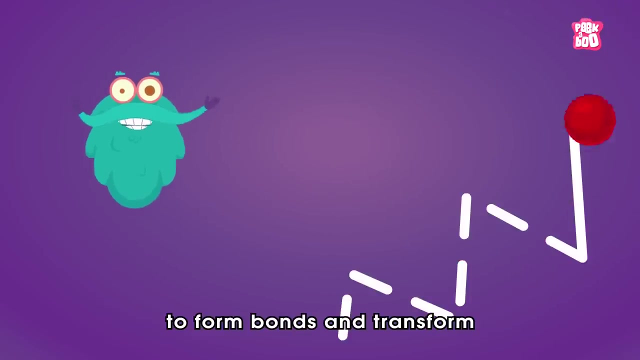 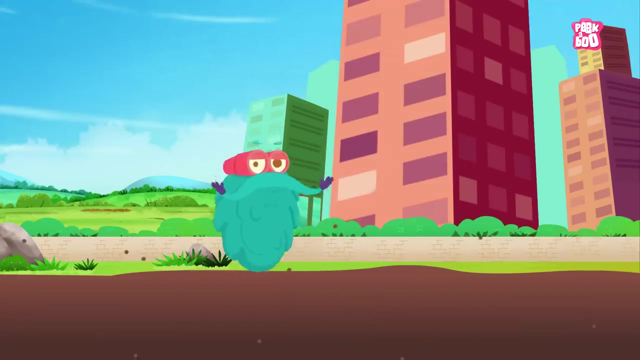 through a process called condensation. That's because when the water is in the form of vapor, every molecule moves so fast in random directions that they find it difficult to align perfectly to form bonds and transform into liquid. So when the microscopic dirt particles like dust on the earth's surface get blown high into the 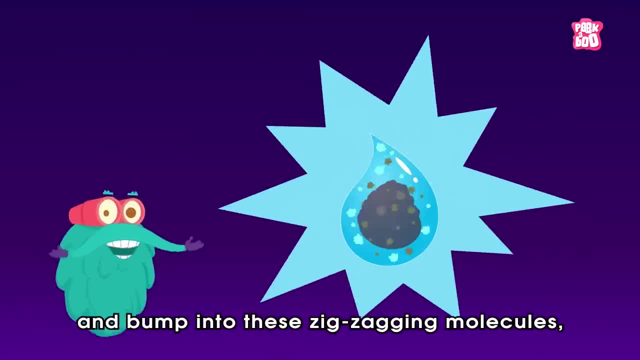 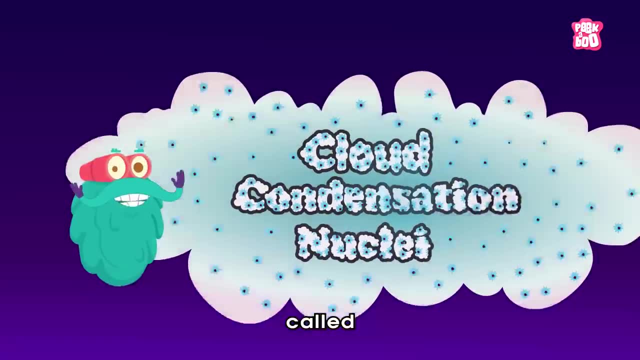 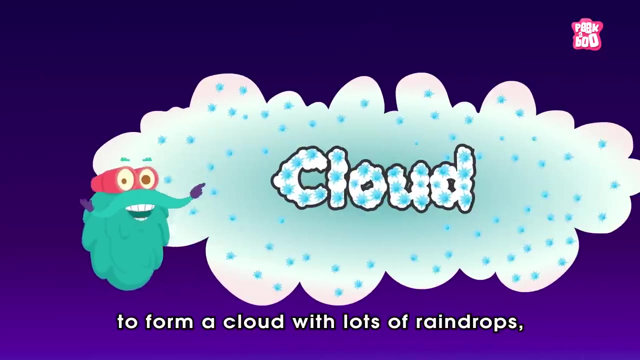 atmosphere and bump into these zig-zagging molecules. the vapor molecules find it much easier to condense around these particles called cloud condensation nuclei. So basically it means to form a cloud with lots of raindrops. we need lots of these nuclei. 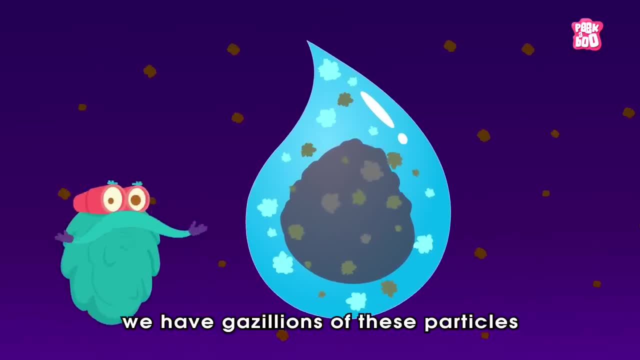 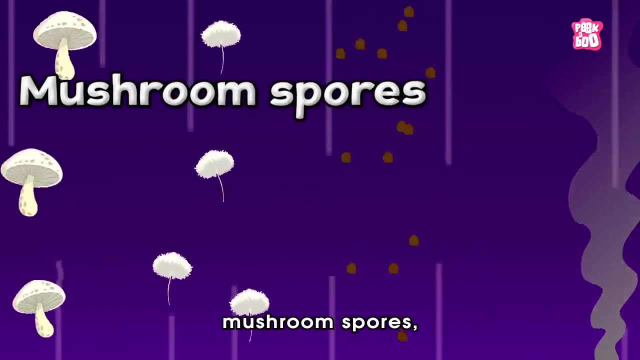 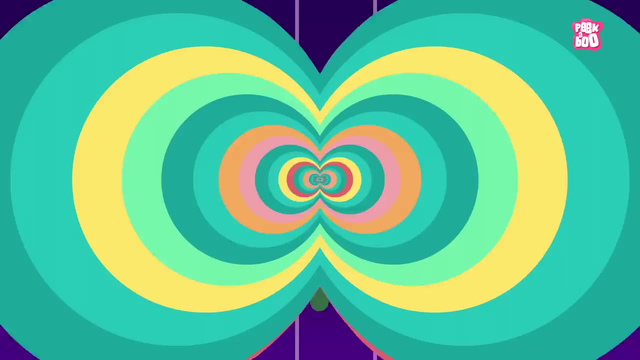 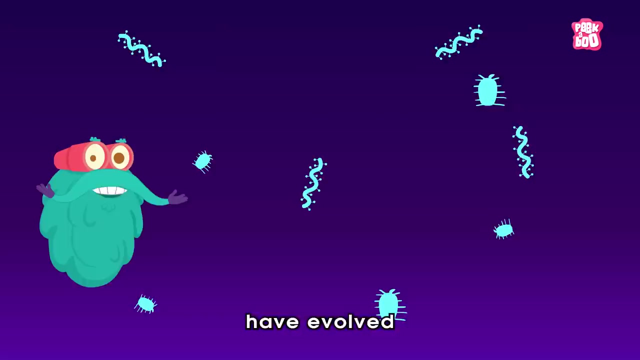 And fortunately, we have gazillions of these particles floating in the atmosphere in the form of soot, dust, pollen, mushroom spores and even bacteria with a name: pseudomonas syringe. Yes, my dear friends, some experts believe that these bacteria have evolved into perfect cloud. 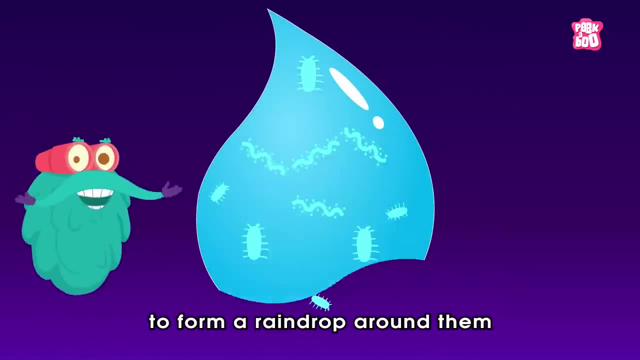 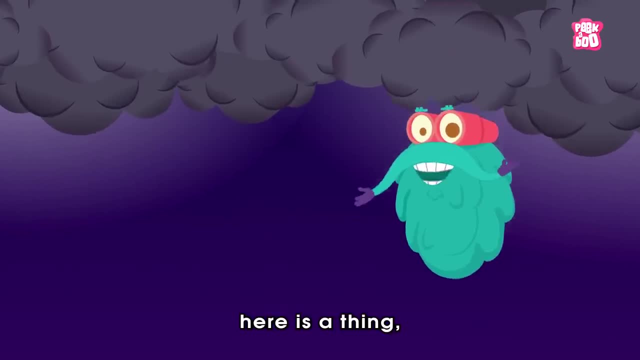 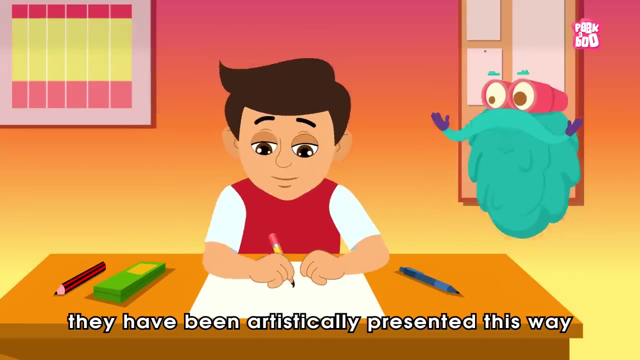 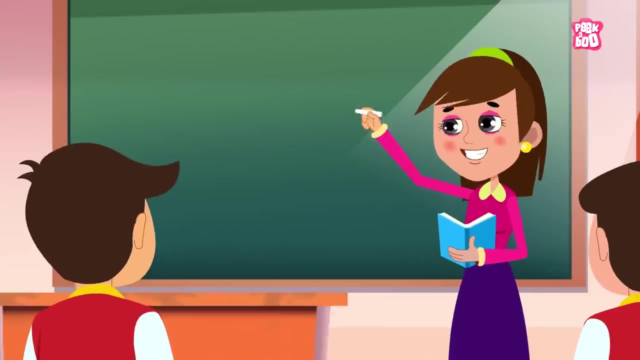 condensation nuclei to form a raindrop around the Earth. them to help the droplets drop down on the ground. and here is the thing: raindrops don't look like teardrops, although they have been artistically presented this way for ages. however, the common raindrop is actually shaped more. 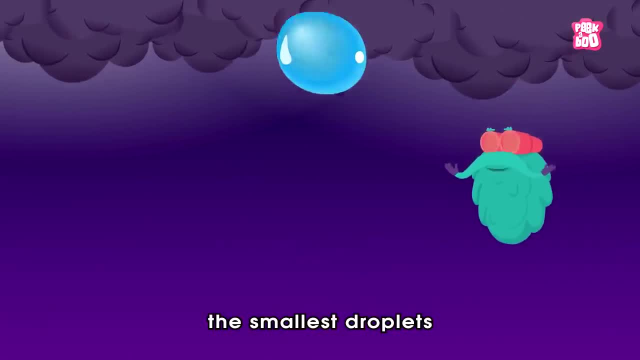 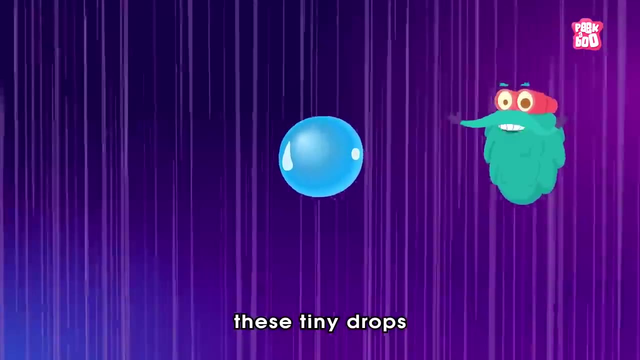 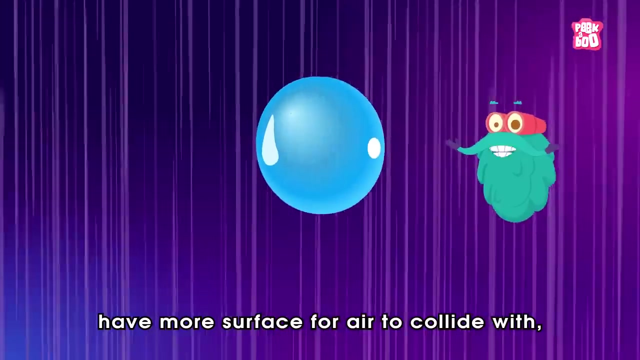 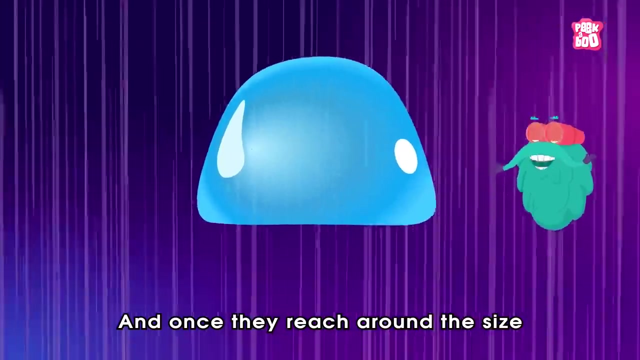 like a hamburger bun. in fact, the smallest droplets start as spheres, but on the way down, these tiny drops bump into each other to form a bigger sphere, and as these larger drops have more surface for air to collide with, they get flat from the bottom and once they reach around the size of five to six, 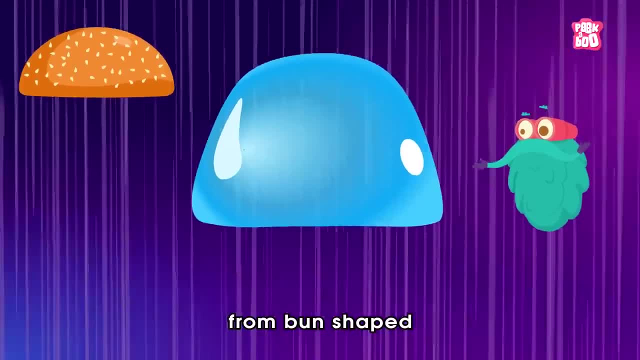 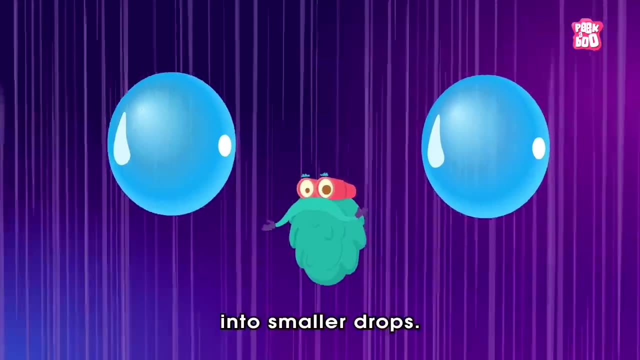 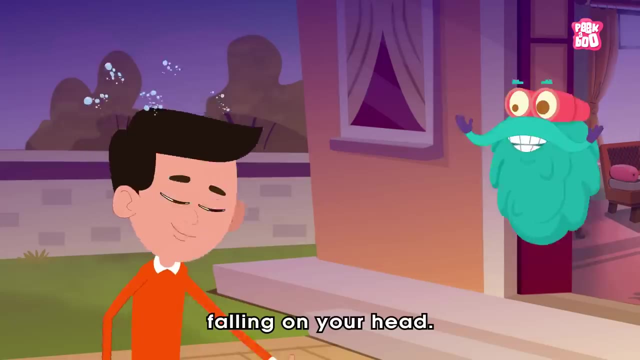 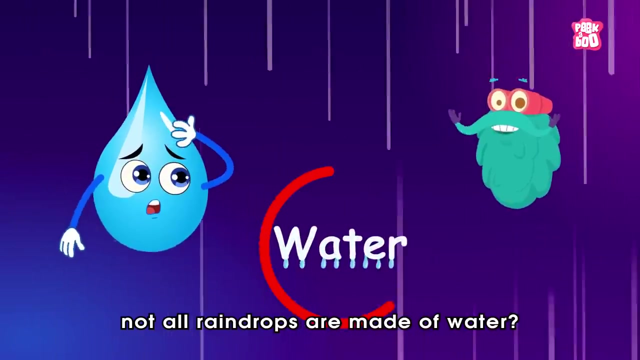 millimeters. they transform from bun shaped to parachute shaped, just to get bigger and bigger, until it bursts apart into spheres, smaller drops, and that, my friends, is a journey of a raindrop falling on your head. trivia time: did you know? not all raindrops are made of water? yes, rain.